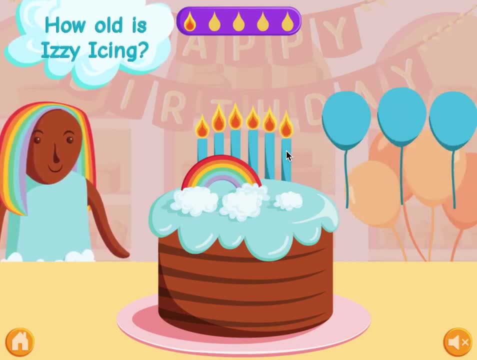 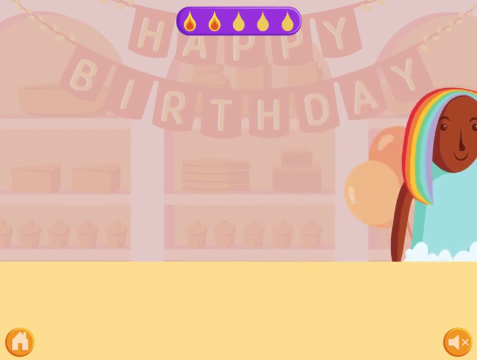 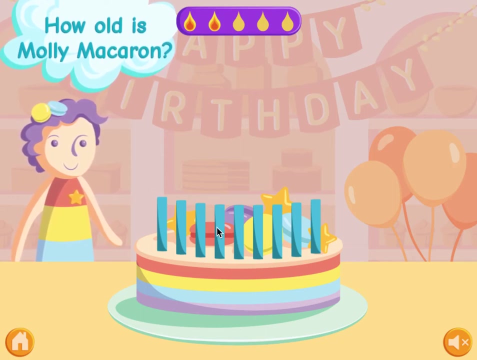 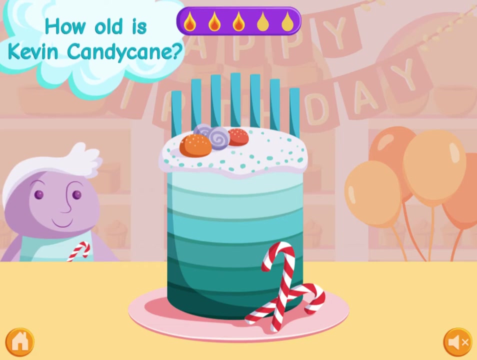 5, 6. How old is Molly Macaron? 1, 2,, 3,, 4, 5,, 6, 7,, 8, 9. How old is Kevin Candy Cane? 1,, 2,, 3, 4. 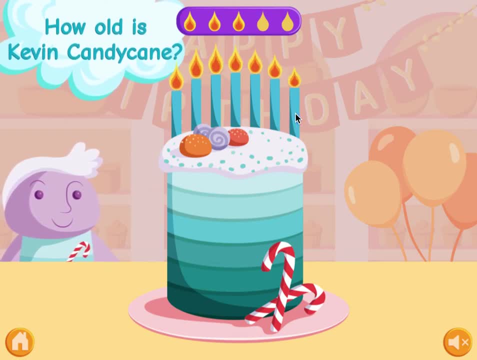 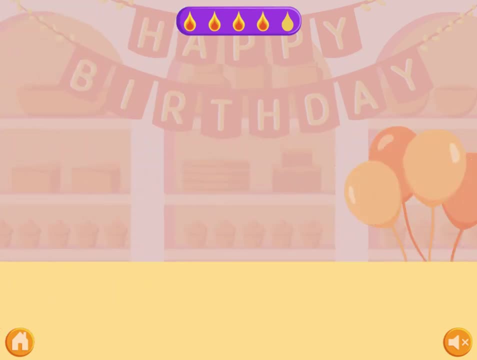 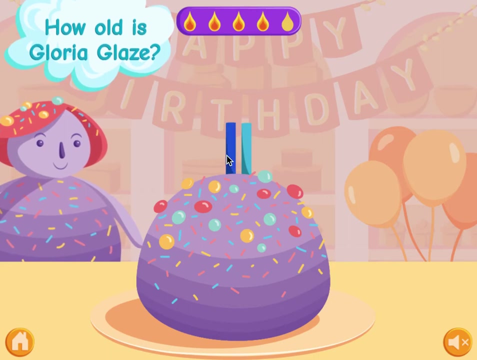 5,, 6,, 7, 8,, 9, 10, 11, 12, 13, 14, 15, 16, 17, 18, 19, 20, 21, 22, 23, 24, 25, 26, 27, 28. 29, 30, 31, 32, 33, 34, 35, 36, 37, 38, 39, 40, 41, 42, 43, 44, 45, 46, 47, 48, 49, 50, 51, 52, 53, 54. 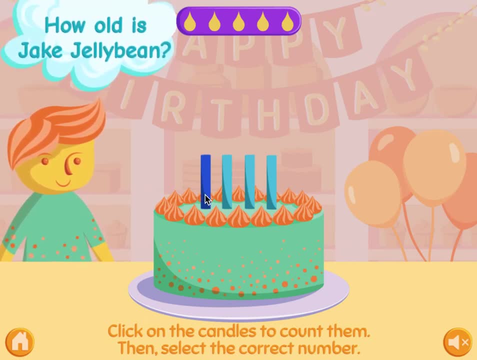 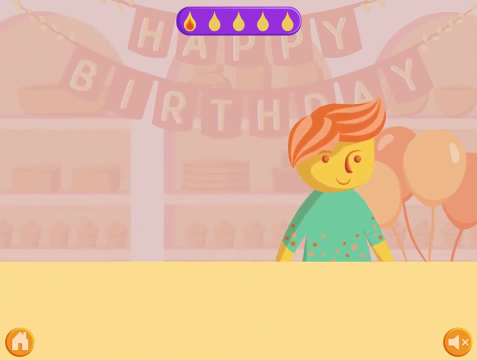 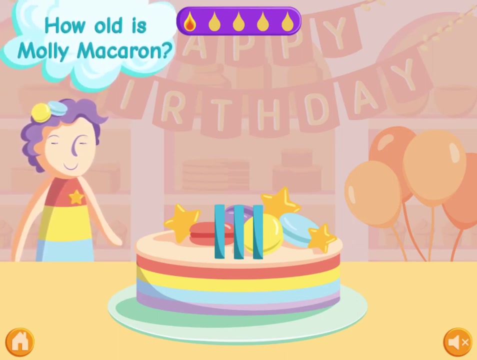 55, 56, 57, 58, 59, 60, 61, 62, 63, 63, 64, 65, 66, 67, 68, 69, 70, 61, 62, 63, 64, 65, 66, 67, 68, 69. 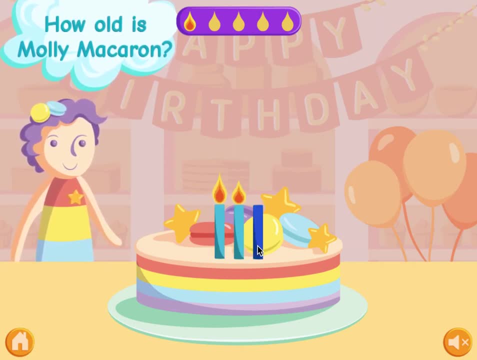 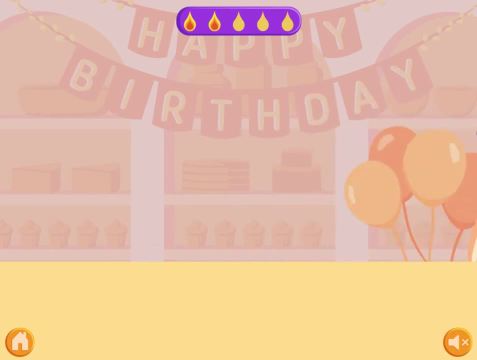 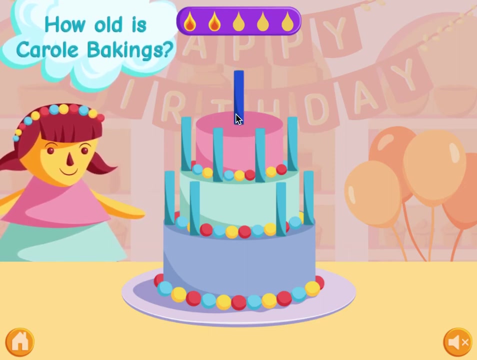 69, 70, 71, 72, 73, 74, 74, 75, 76, 76, 77, 78, 89, 90, 91, 92, 93, 92, 93, 94, 95, 96, 97, 98, 99, 100. 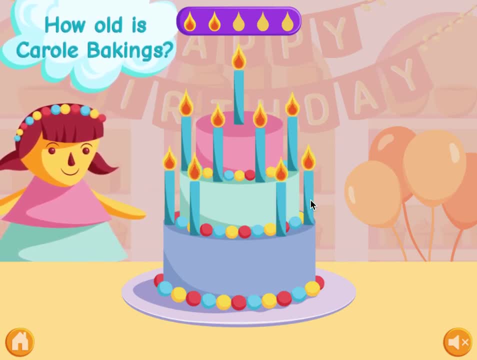 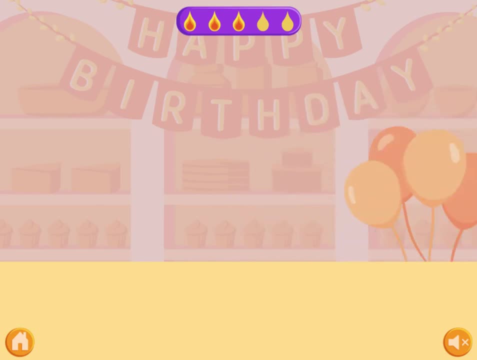 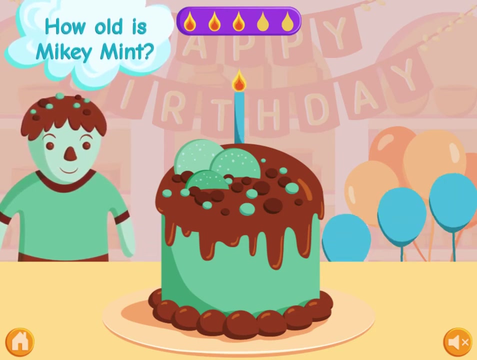 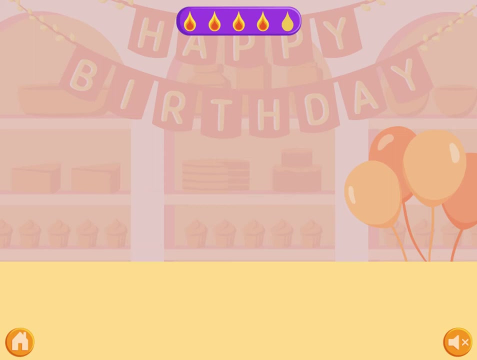 100: 12, 13, 14, 15, 16, 17, 18, 19, 20, 21, 22, 23, 24, 25, 26, 27, 28, 29, 30, 31, 32, 33, 34, 35, 36.